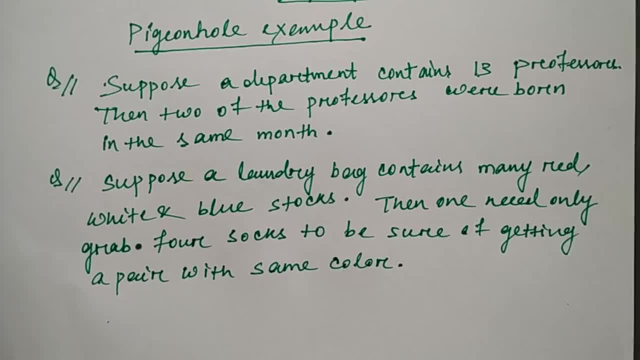 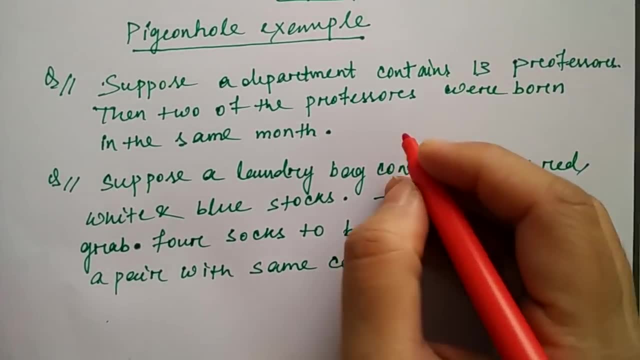 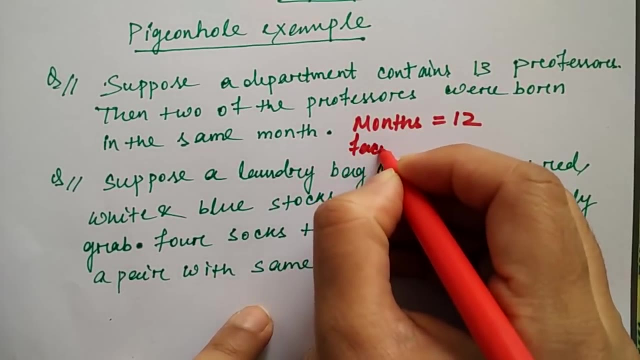 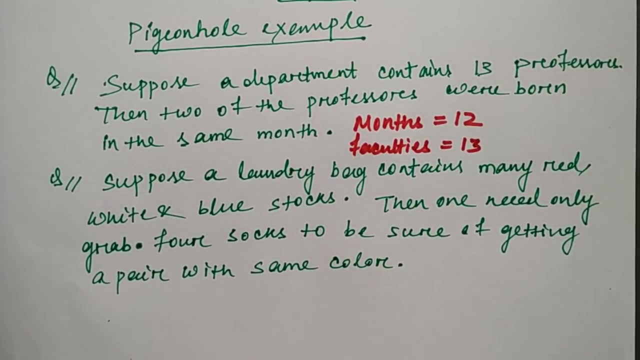 what? 13 faculty and two of the faculty were born in the same month. so, totally, how many months are there in a year? number of months are 12, right, and how many faculties are there? faculties are in 13 number, so the at least chance is, let's say, if 12 of the faculties are born in different. 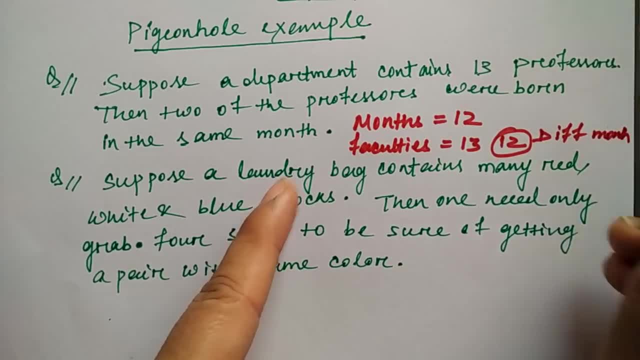 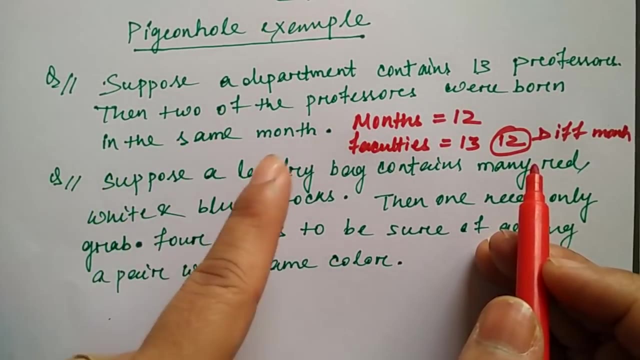 different month, right? so where is that one more faculty will go? that faculty is also born out of the any 12 month, right? so one of the month is getting repeated and other 12s are same. that is why it is told that two of the professors were born in the same month, which is giving a condition. 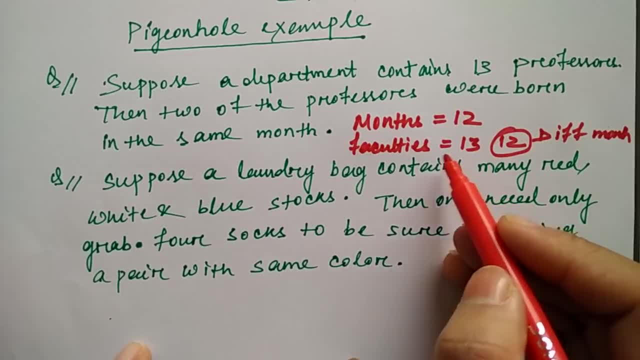 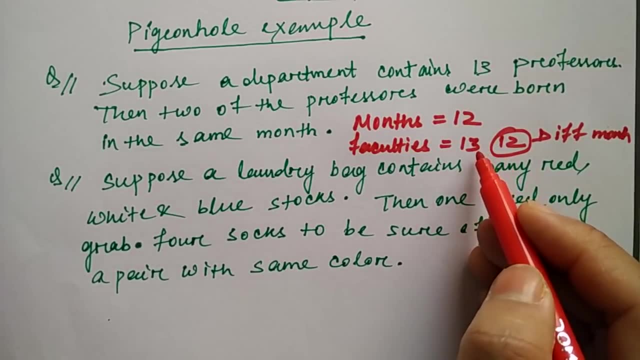 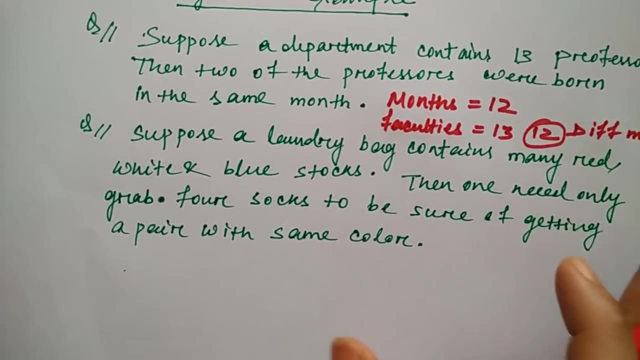 of peasant hole. you understood. if you say that the faculties are peasants and month are peasant hole, then you will understand that one peasant hole is having more than one peasant. or you can say faculty, one month is having more than one faculty. here what it is saying in this one? suppose the laundry wear contain many red. 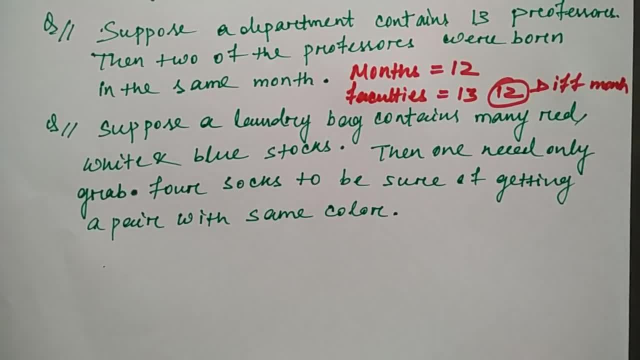 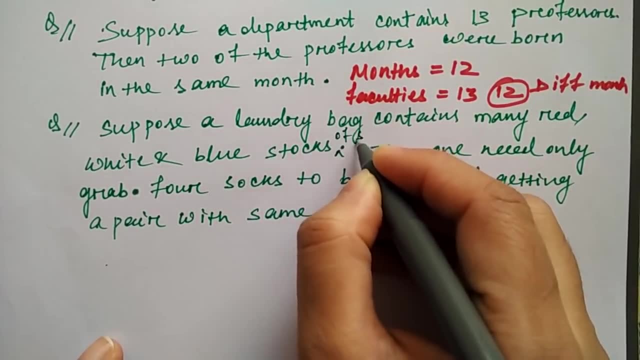 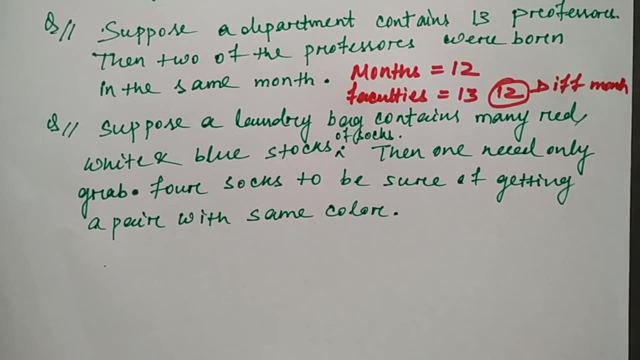 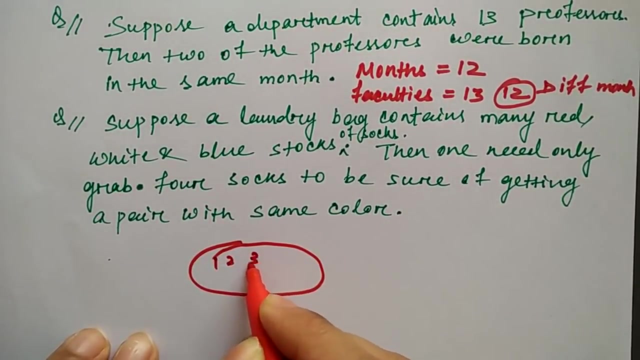 white and blue stocks. okay, so stocks of socks, actually stocks of socks. okay, so many socks are there of blue, white and red color and the need of grabbing four socks to get a shot of two same color. so it is saying that you have collected. let's say, this is the laundry bag and here different socks are there: one, two, three, four. 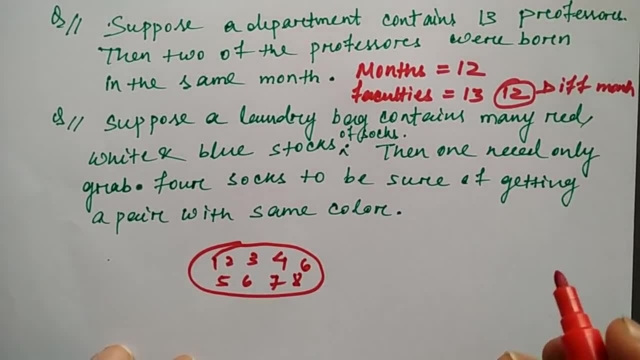 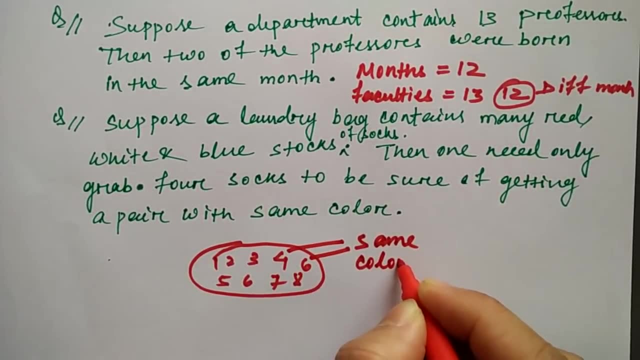 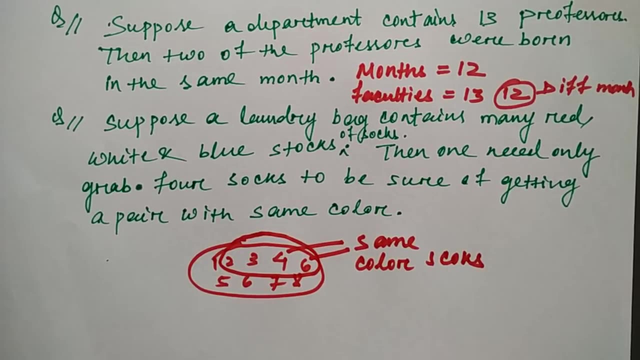 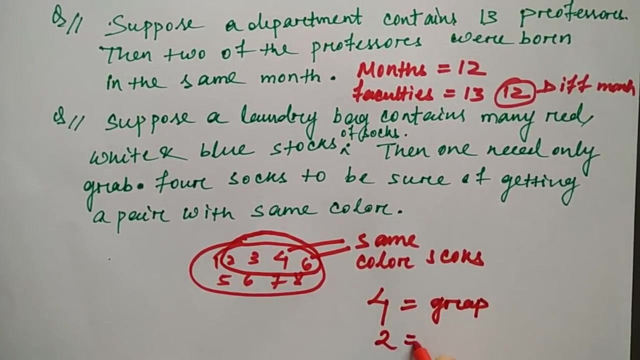 five, six, seven, eight, many different, and all are of different, different color. so it is asking that to get two same color socks, same color socks, you should grab four at a time, right? so what it is saying, when you are grabbing four socks, four socks, you are grabbing and getting two socks of same color, but there are three different color colors. are 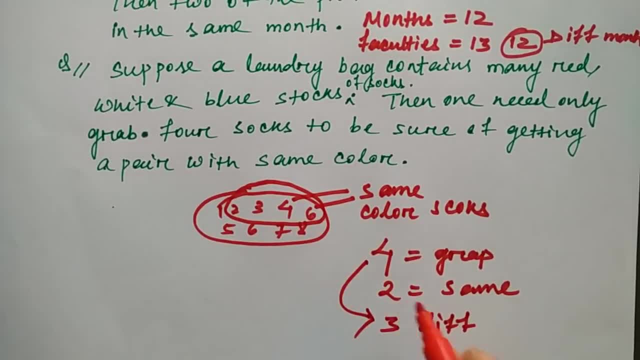 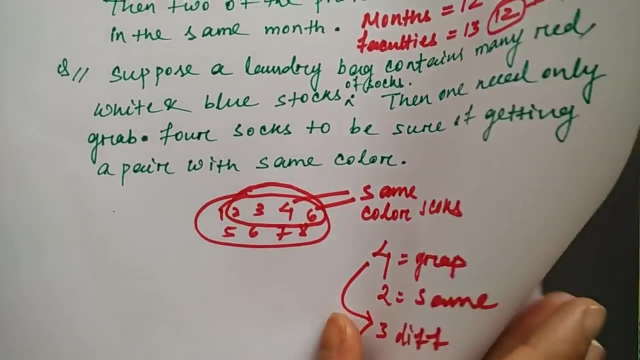 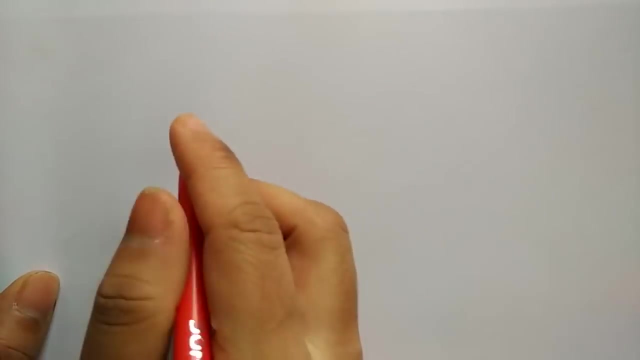 three different right. so when you are getting four, one, two, three will be of three different color, but the other one is same with any of that. so this is why it is giving the condition of pigeonhole. we'll see some problem. there is a formula regarding the pigeonhole. if you have got. 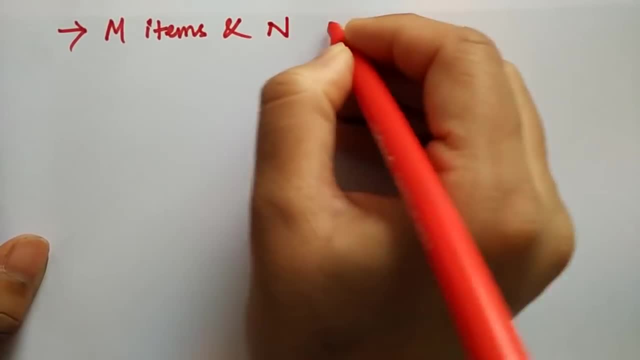 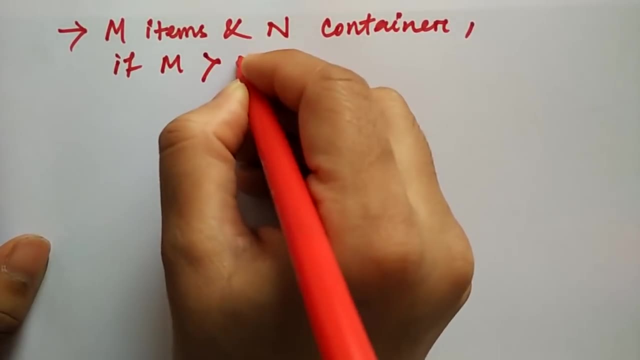 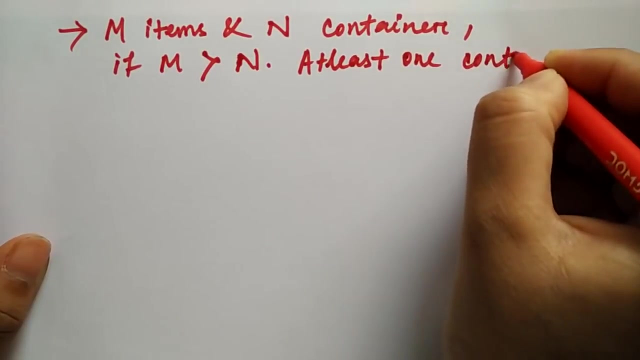 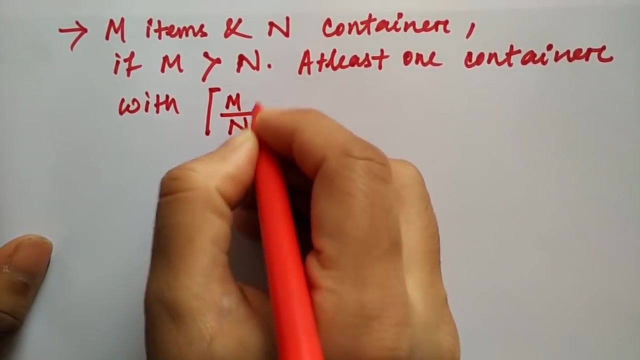 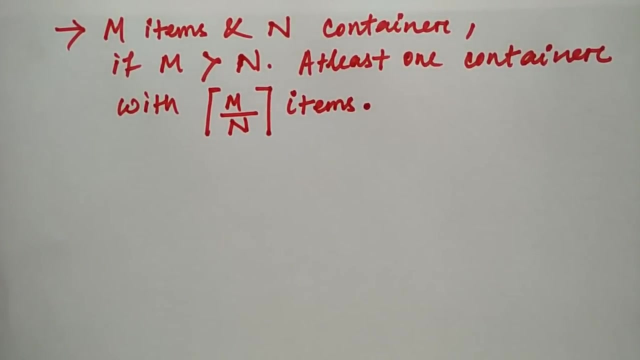 m items and n container and if m is greater than n, then at least one container with m divided by n sealed items. so if you have got m item and n container where the number of item is more than the number of container, then one container will be having m divided by n sealed, at least one, it is not. 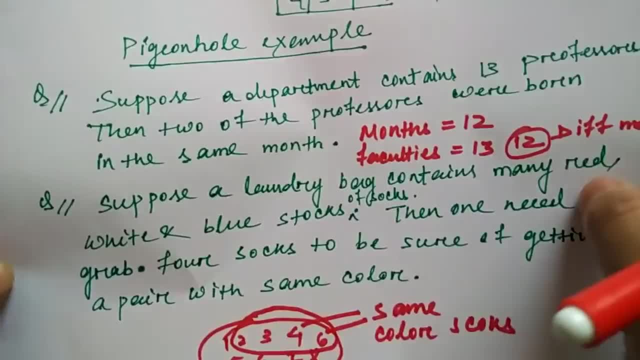 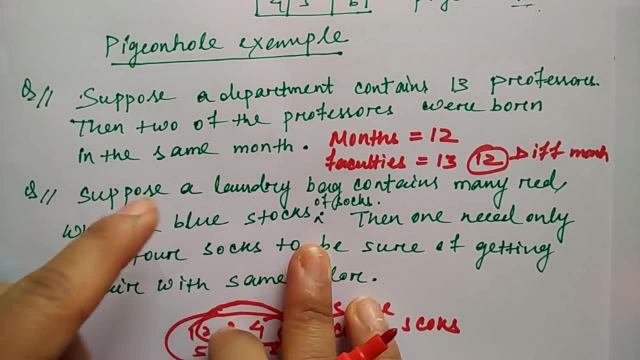 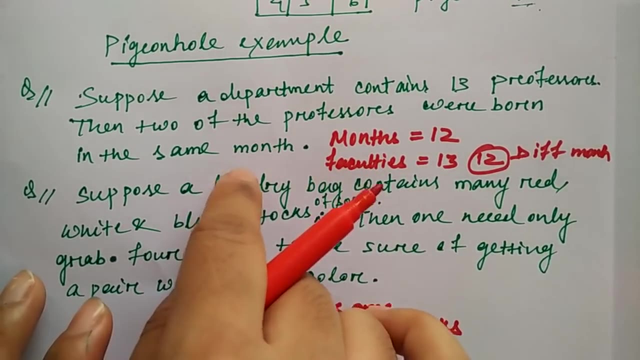 not saying than more. so will take the same example of the previous one, that to show that how it is containing in a particular month to faculty, he has told the total 13 faculty or professor are there and two of the professors were born in the same month. so how can you prove that it is correct? 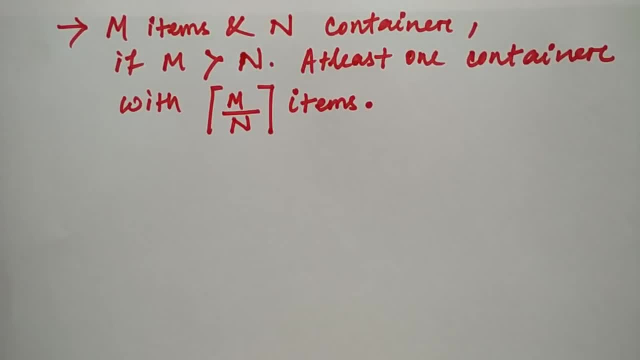 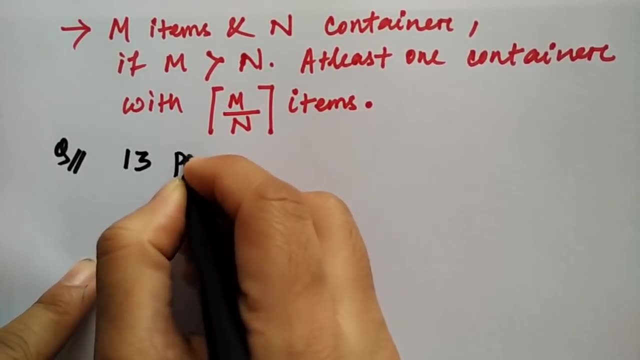 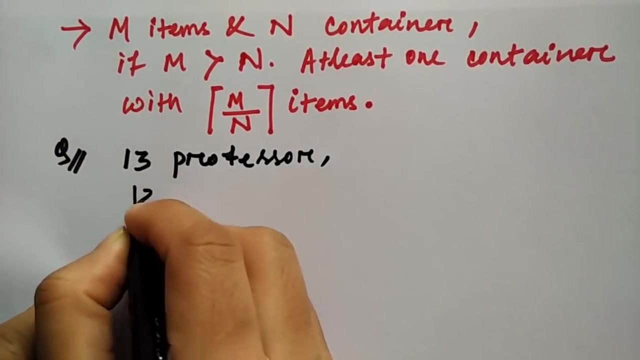 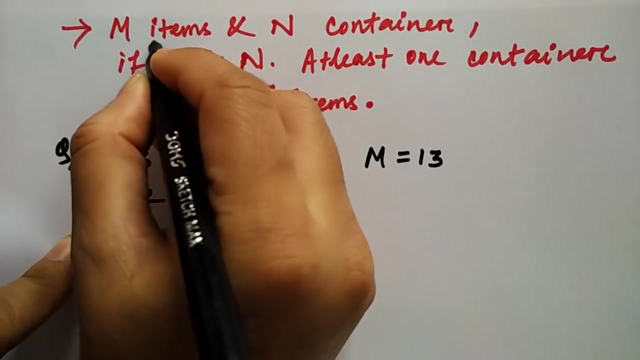 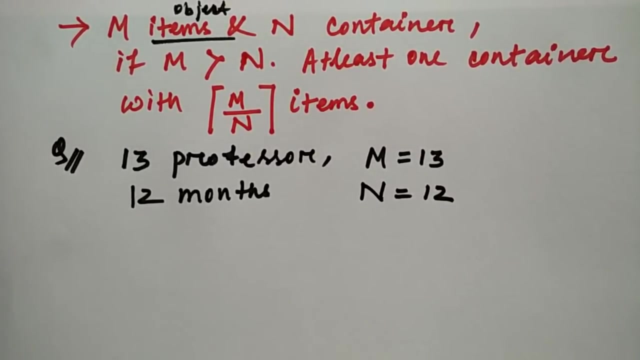 by using this formula, so i will show you how to do it. let's say like: according to the question, we had 13 professor and 12 month. so here item will be the professor or item or any object you can see that is leaving or non-living, and container is month. obviously, because we are determining depending upon the 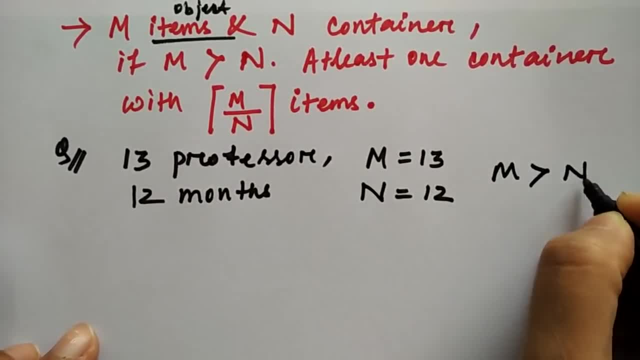 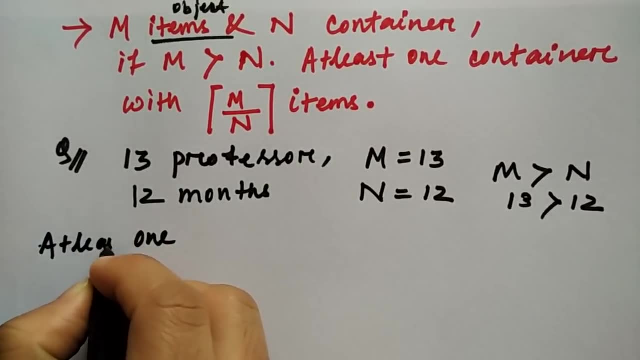 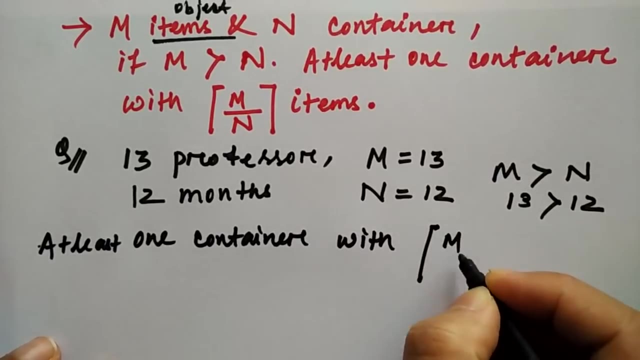 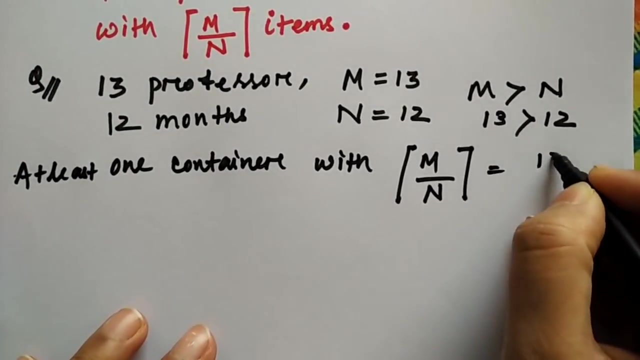 month. so m is greater than n, it is justifying 13 is greater than 2. then at least one container, at least one with m by n seal. so what is m by n here? m by n is 13 by 12. see, so this value will be.